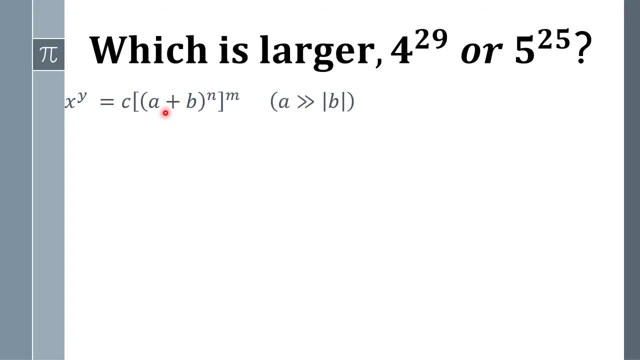 a must be positive, b can be either positive or negative, but a has to be significantly larger than the absolute value of b. We try to use the first few items of the expanded expression to estimate the value of a times b to the n-th power. 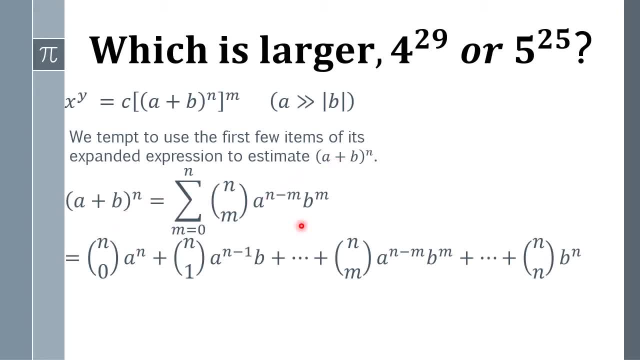 This is the expanded expression. The first two items are most commonly used, but sometimes we might need to go further to have a closer estimation. The key to success is to carefully choose a, b and n so that a over bn goes as large as possible. 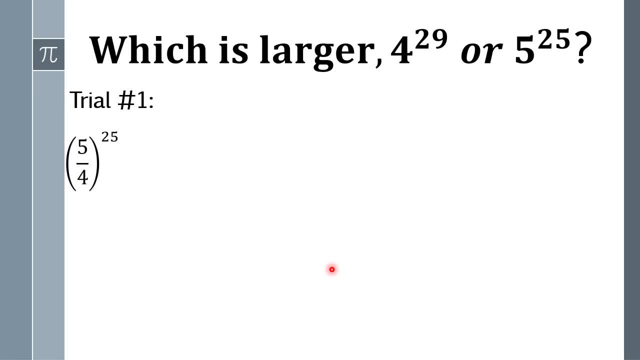 Let's give it a try. The most simple way is to write 5 over 4 as 1 plus 1 over 4.. However, in this expression the value of a over bn is very small. That means we will not be able to use a few items to estimate its value. 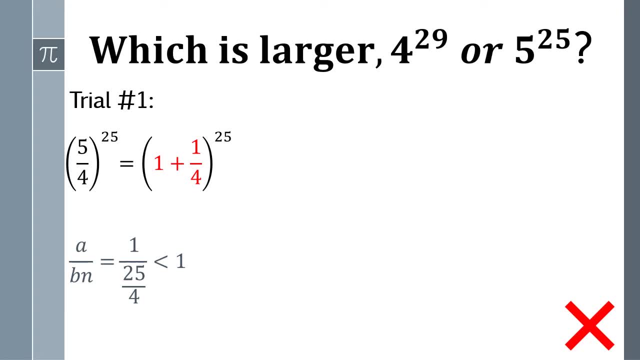 It's a no-go, Let's give another try. We can write 5 over 4 to the 25th power, as 5 over 4 to the 5th power, then to the 5th power, And the inner side can be written as 31, 25 over 10, 24,. 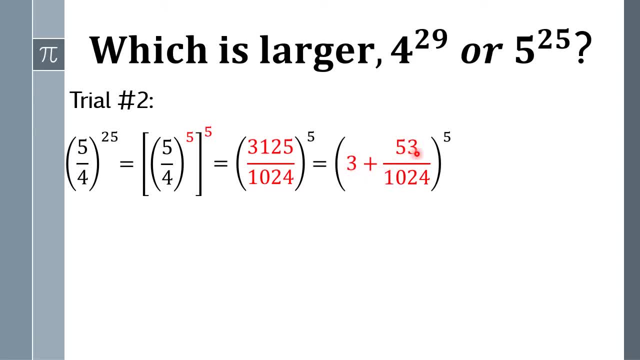 which is equal to 3 plus 53 over 10, 24.. Let's calculate its value a over bn, which is larger than 10.. That's good enough, Let's continue. So here we will use the first two items. 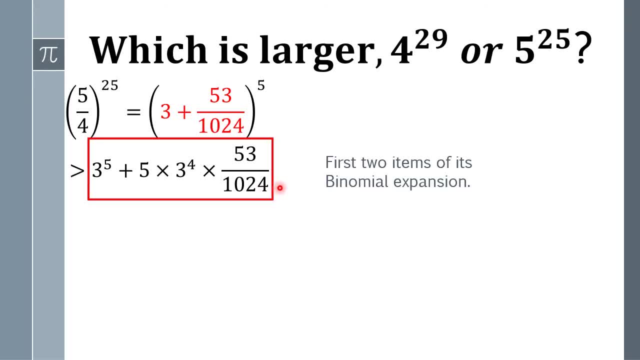 to estimate the value, And apparently there is a larger than signal here. However, 53 over 10- 24 is still not easy to calculate, but we know it is slightly larger than 0.05.. So we use 0.05 to substitute 53 over 10- 24.. 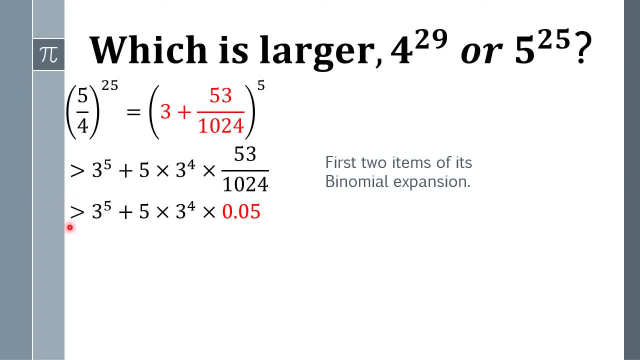 And again there's a larger than symbol here. The calculated value of this expression is 263.25,, which is larger than 256.. Or we can say 4 to the 4th power. So we have proved that 5 over 4 to the 25th power. 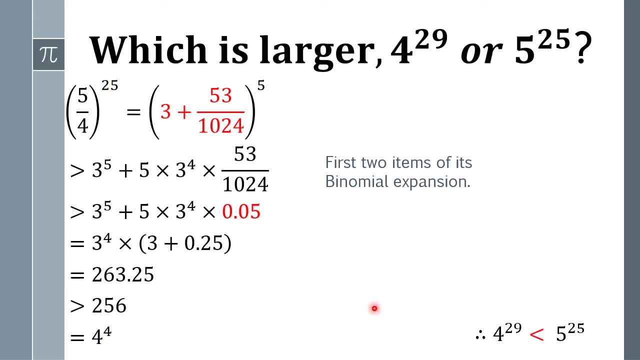 is larger than 4 to the 4th power- And eventually you can get 4 over 29- is smaller than 5 to the 25th power. We want to explore if there's another way. So here is trial number 3.. 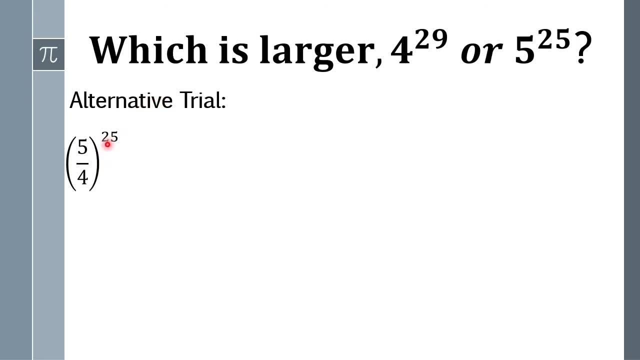 We know 25 is equal to 1 plus 3 times 8.. So the entire expression can be further written as: 5 over 4 times 2 minus 3 over 64. to the 8th power, And to calculate the value of: 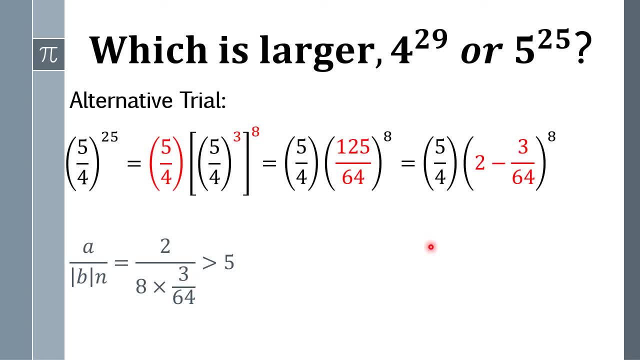 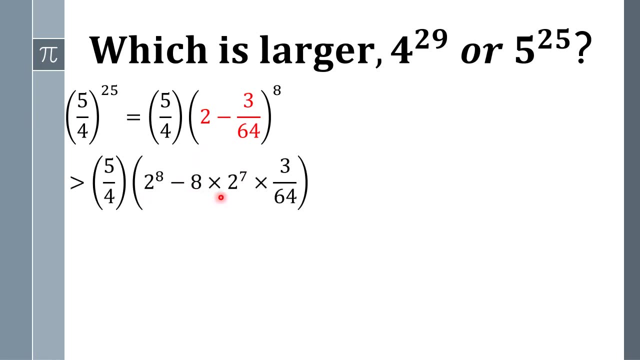 a over b, n is larger than 5.. Probably good enough. Again, we will use the first two items of expanded expression to estimate the value which is shown here, And the calculated value of this expression is 260, which is larger than 256.